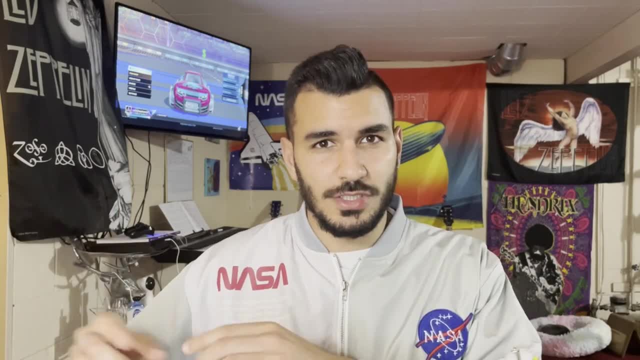 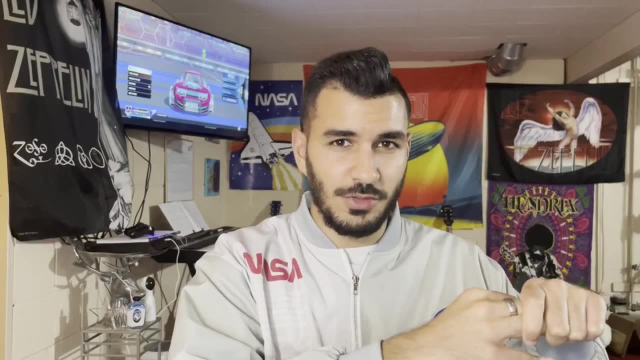 it and apply it to communication systems Generally, for example when you're modeling noise in a system. So if you really struggle with probability statistics, then you struggle with the applied electromagnetics, you struggle with the frequency domain, stuff from signals and systems- and you put 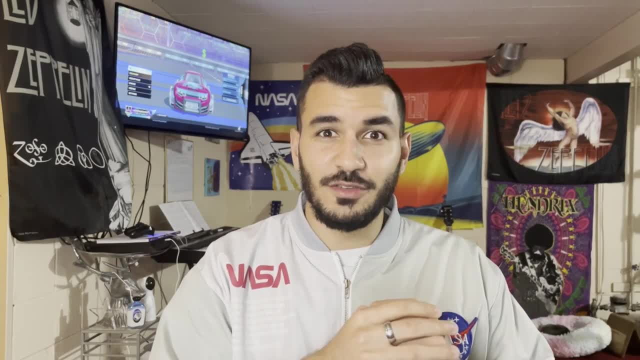 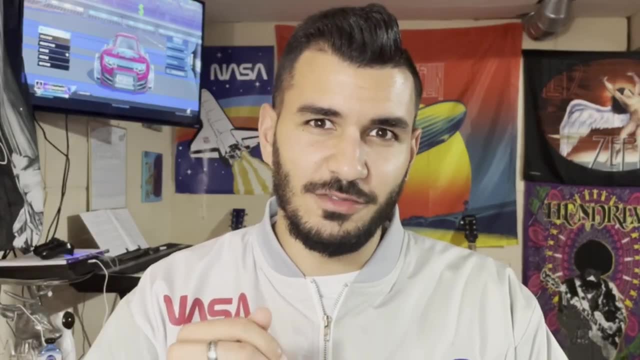 all that stuff together in communication systems. that class is usually a nightmare for a lot of students. And the funny thing is I taught that class twice as a teaching assistant And although I really enjoyed teaching it and I had a lot of fun teaching it, teaching that class just helped. 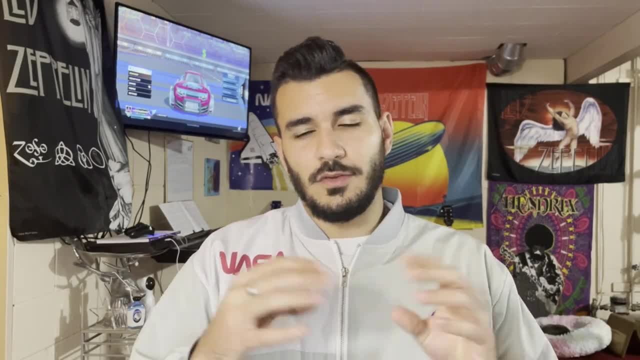 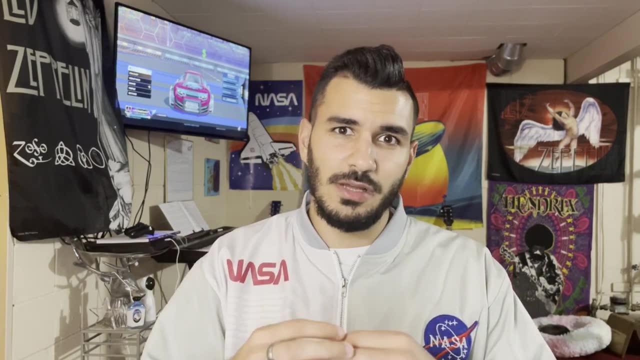 me understand the magnitude of how confusing all this stuff is. The fourth most difficult class, I would say, is Microelectronics, And that's where you start learning about transistors and how to take transistors and build amplifiers with them And you start having really complicated circuits. 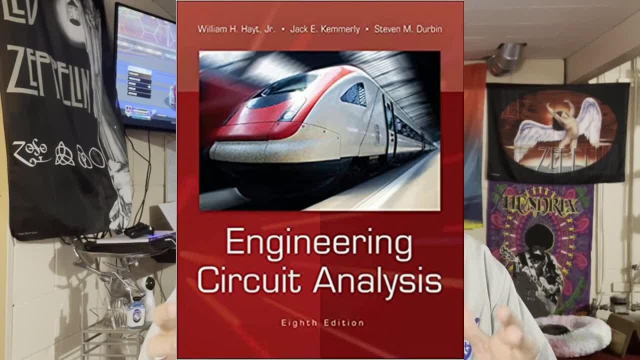 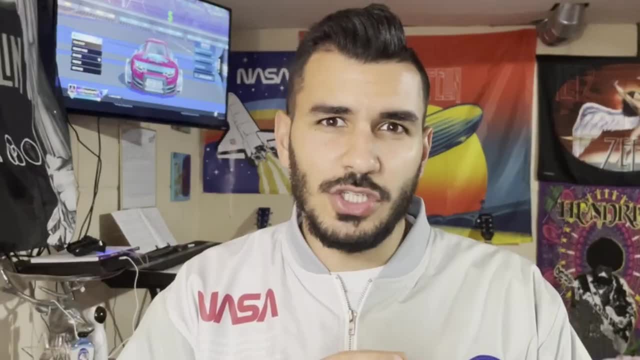 Now the introductory course to that is Circuit Analysis. And Circuit Analysis is pretty simple because you basically learn about like resistors, inductors, capacitors, put them together in networks and you have like a bunch of equations where you solve for like one variable generally. 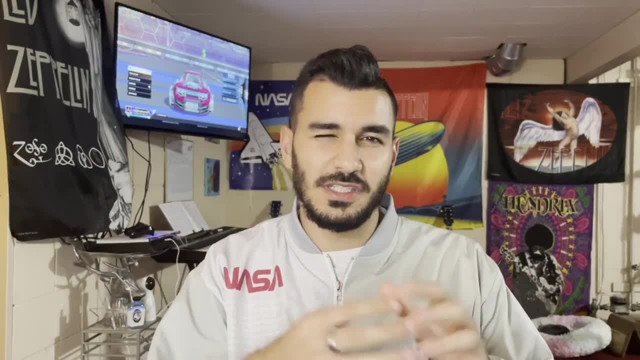 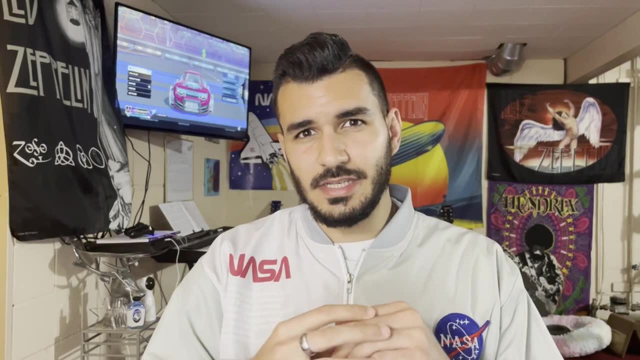 And even if you don't know what's going on, you can still do fine in the class because the math is a lot simpler. Now, the fifth hardest class I would say is Embedded Systems, slash VHDL, And I group these things together even though they're different. 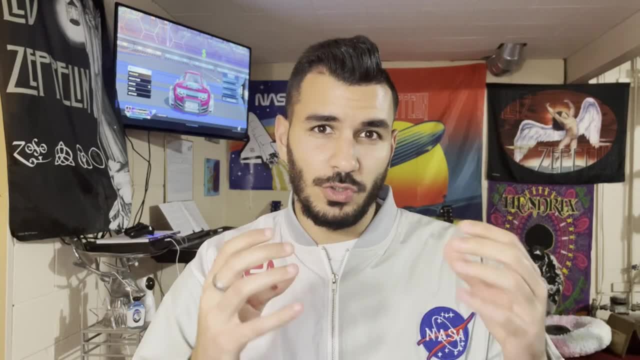 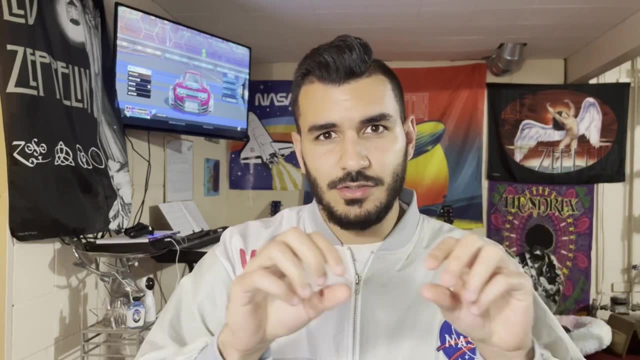 Because they kind of are trying to achieve similar things, where in Embedded Systems you're working with microcontrollers and you're usually doing some type of program like Arduino or some type of microcontroller in which you are typing lines of code and software in order to achieve some. 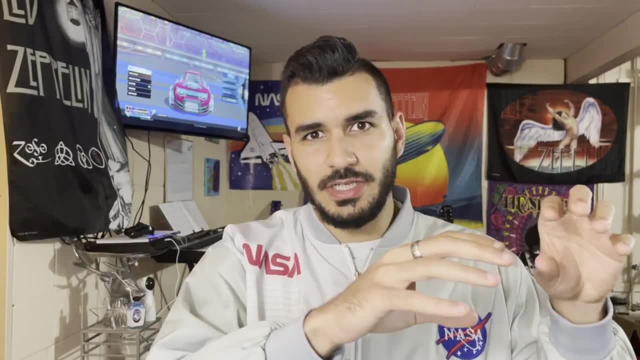 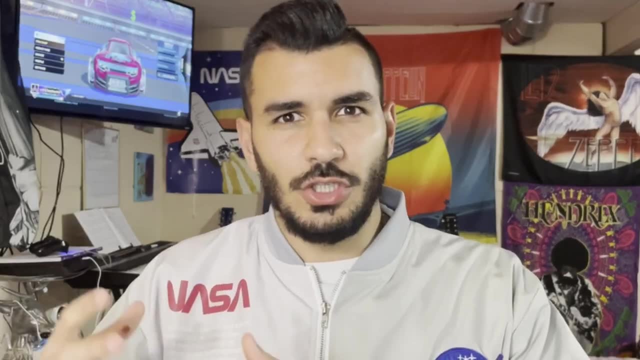 outcome in hardware And a very simple example of that is like, for example, writing like a piece of code that makes an LED blink or makes an LED have like a I don't know. it can make like a clock or an alarm, And this is generally where a lot of students can tinker and build projects And a lot. 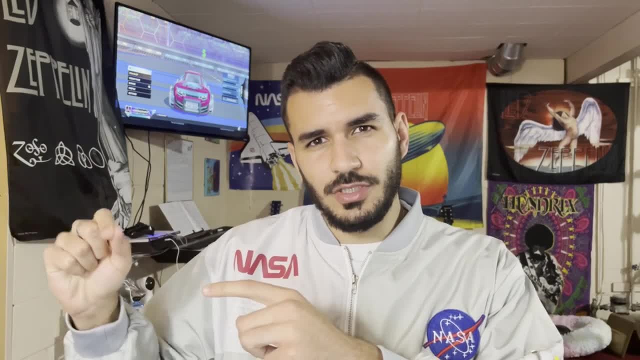 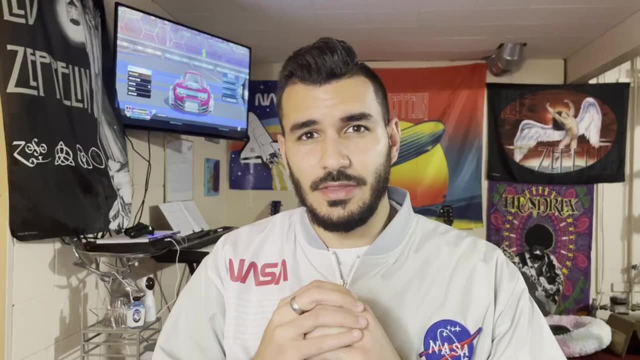 of senior design projects are usually in this area. Now VHDL, which is a little more difficult, also aims at the idea of like programming hardware, although you are doing it directly through like logic gates and ALUs and things of that nature. So VHDL is harder, but I 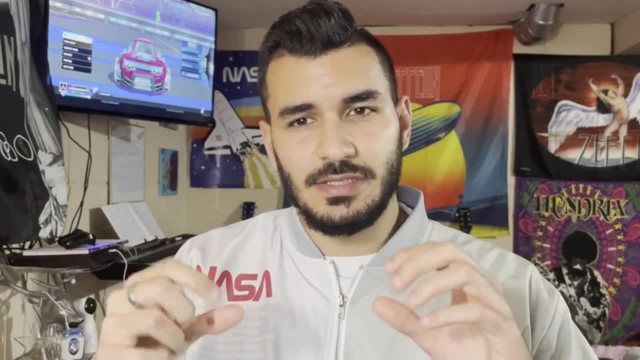 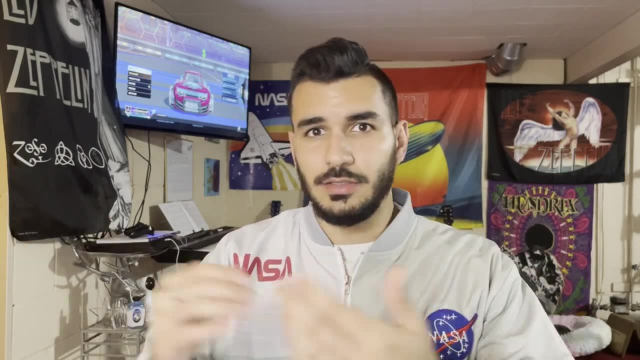 would group Embedded Systems and VHDL as easier than the other stuff because it's like more hands on applicable. you get to like program and play around with stuff, which is more fun, And you get to actually see the result and learn from trial and error versus some of the class that more. 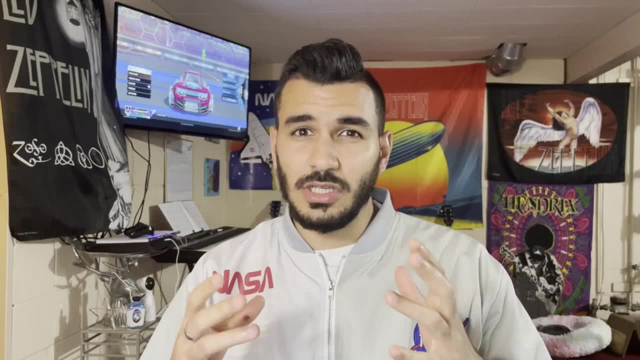 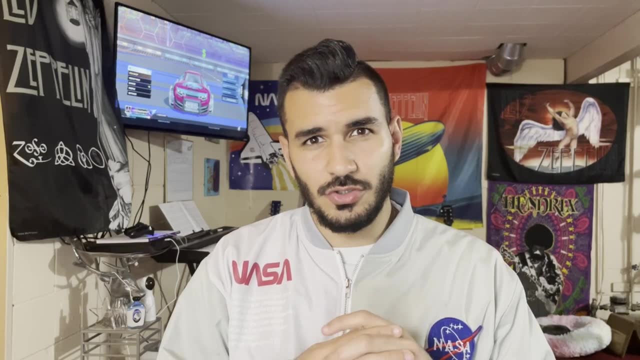 difficult classes I mentioned earlier are generally very theoretical, which can make it really hard to understand what's going on Now. the next class after that is digital principles, And generally it's an easier class because it's an introductory course to basically how binary numbers, binary systems, how binary numbers work, why we use binary, why computers. 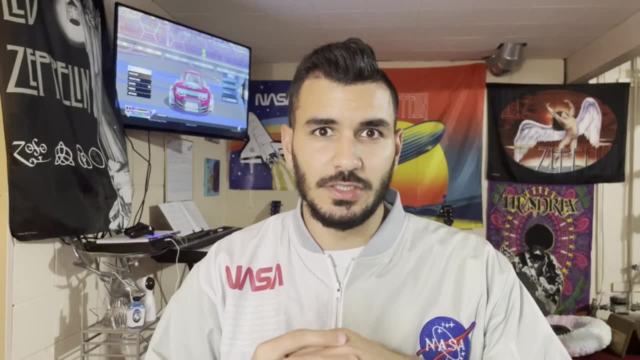 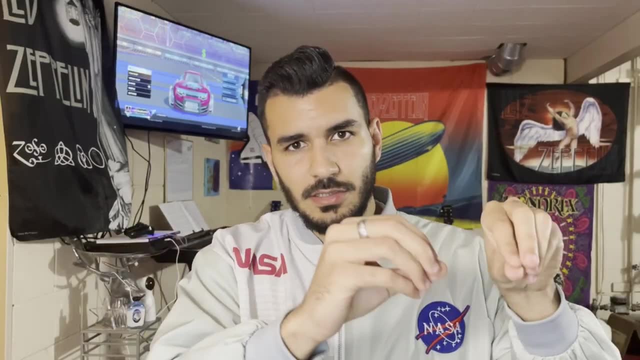 use binary. This is really like the foundation of like computer engineering, where you start building logic gates and you start doing some basic things And you can like, for example, understand how a calculator is built and you understand how these little binary logic gates. 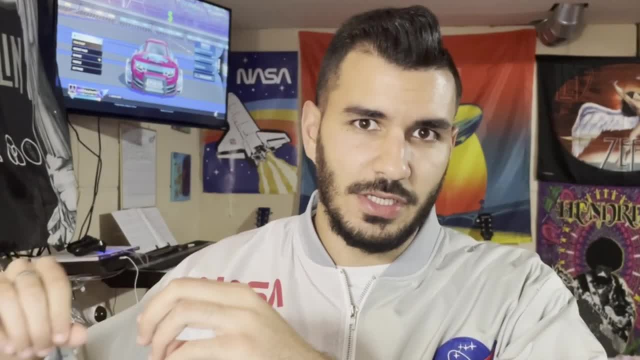 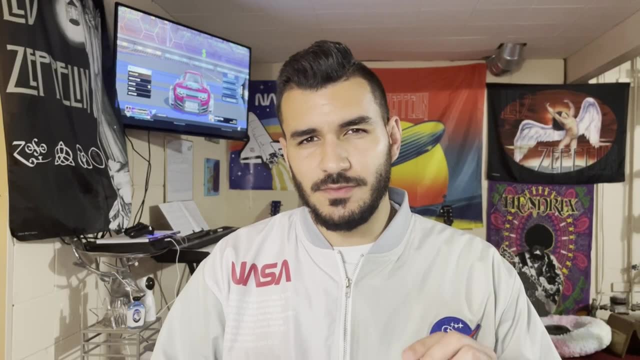 are basically the fundamental building blocks of things like processors and RAMs and basically all the fancy digital circuits that you see in your computer. Now, the nice thing about this course is it starts from absolute scratch and it's very logical and does not have like intense mathematics. 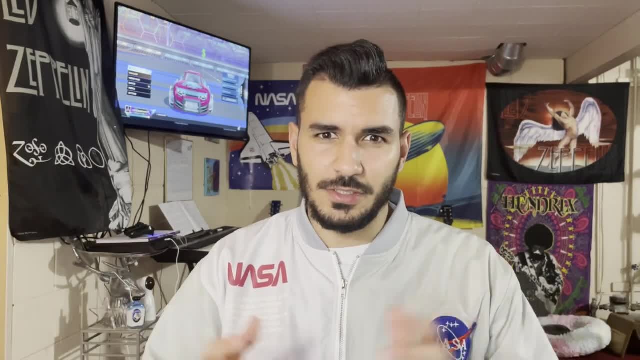 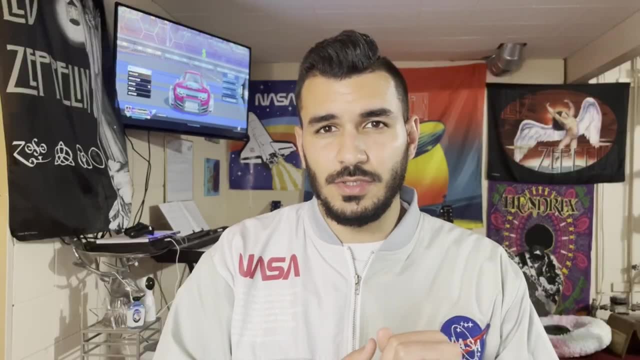 or anything. It's pretty straightforward, So, as long as you just keep up, should be pretty easy. Last course here, and in my opinion the easiest- is energy slash power systems And one thing that makes this course easier than the previous ones, even though it's still very theoretical, and 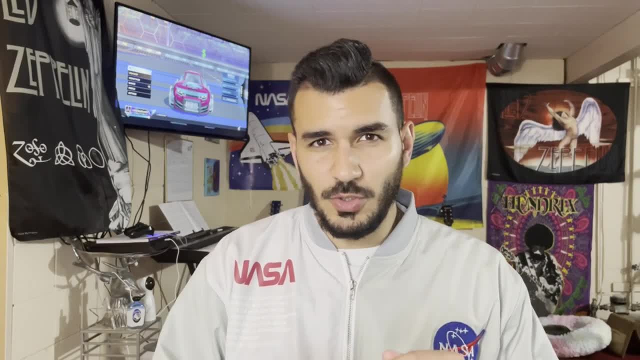 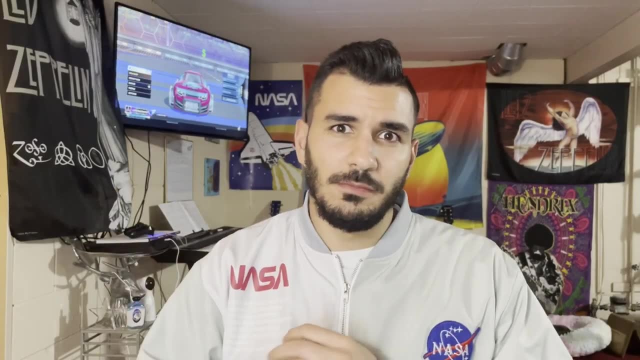 rigorous is the simple fact that you're dealing with like large numbers rather than small numbers. For example, with communication systems, you're dealing with like really, really tiny powers like picowatts, But with energy systems, you're dealing with like megawatts, gigawatts and really. 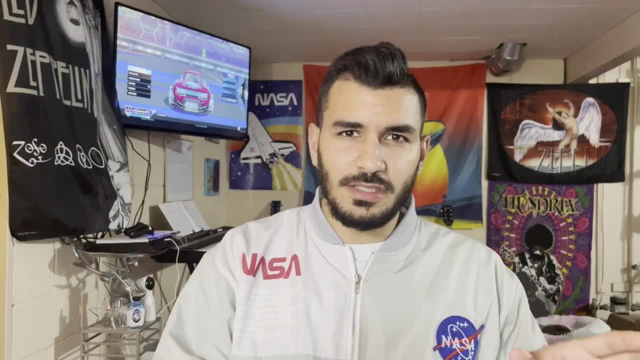 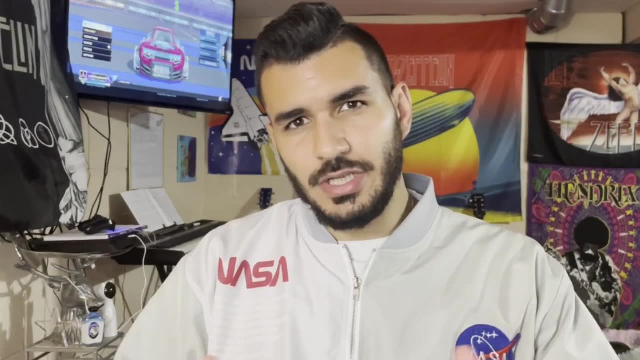 high numbers, So that makes things easier to visualize. But what actually makes this class easier than the others as well is the idea that energy systems, at the end of the day, are really all about like efficiency. You're like generating energy from some source and you're trying to 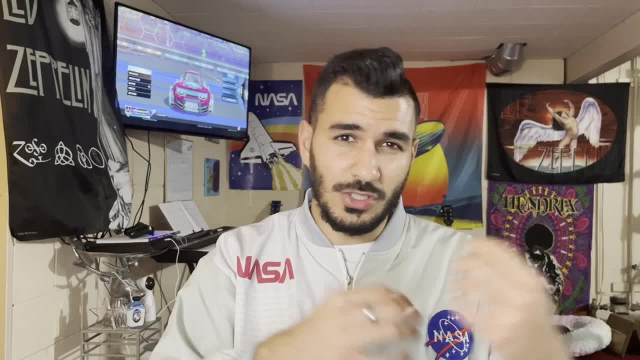 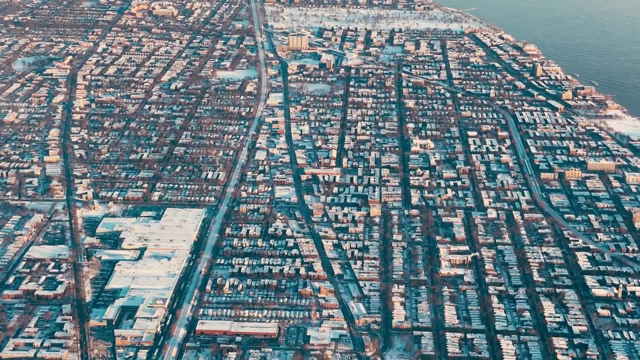 transport it through like some type of cable. You're converting power from one source to the other And you're basically trying to do that as efficiently as possible. And now you take that power and you're distributing it across, I don't know like a city or a town or whatever, or like 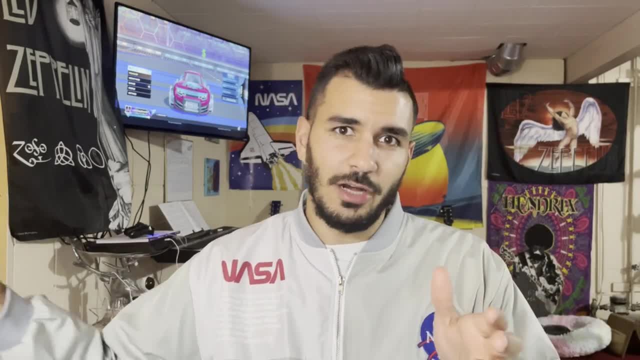 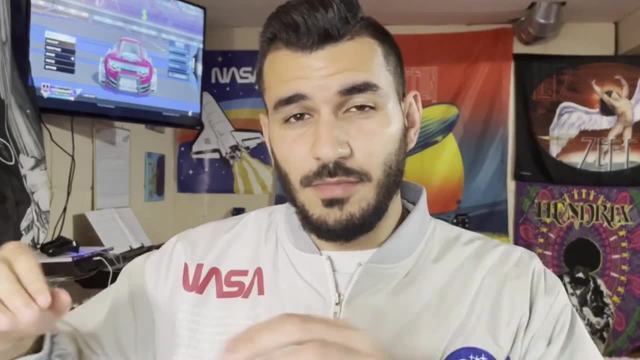 a car or something. It's really all about how you efficiently distribute that power. So the fundamental concepts are pretty straightforward. Now, generally, this has been my observation from being a student and a teaching assistant. But for me, actually, if I were to list these courses from: 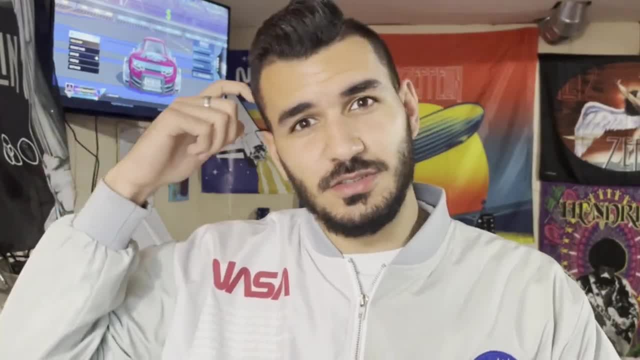 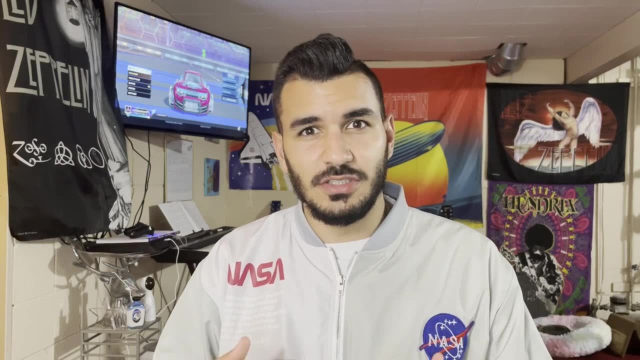 easiest to hardest. I would actually flip this table upside down. So, power systems. when I took that undergrad, that class, it was really hard for me to even just show up to lectures and actually understand what's going on, because I was just not very interested in the concept And on the other, 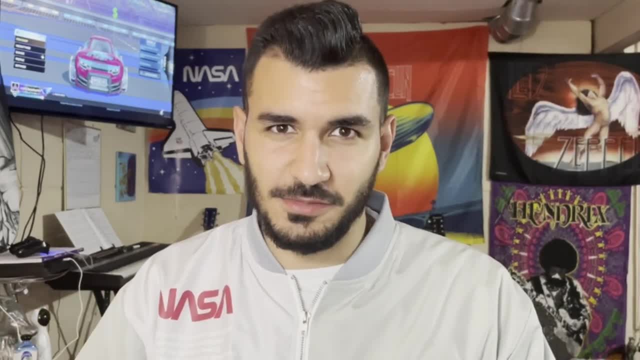 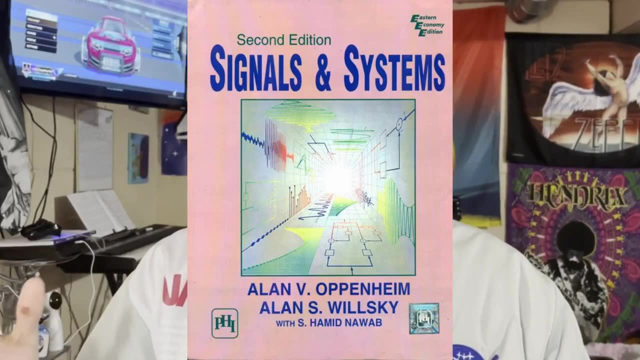 hand, I was completely fascinated with signals and systems and communication systems. I remember when I would carry around my signals and systems book- it was like this pink book And I would just carry it with me everywhere just because it was so fascinated by it. And that's actually when I 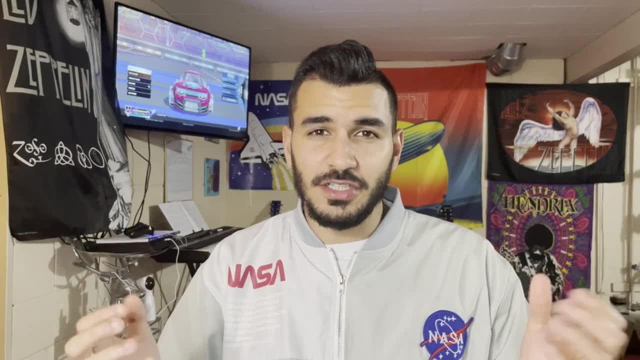 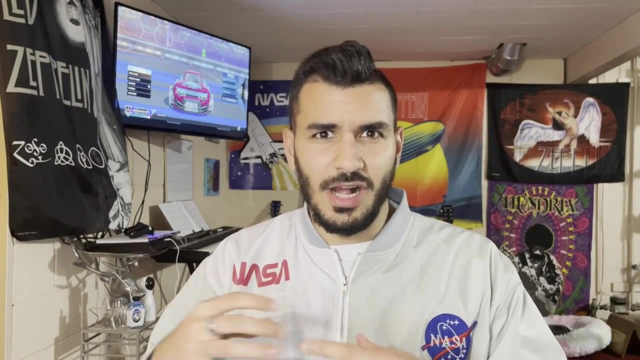 came to realize that the definition of easy and hard for most people vary. Some people categorize hard and easy by like rigor, difficulty, or by how hard the concepts are, or like how abstract it is. But for some people, including myself, hard and easy really just depends on how enjoyable or fun.